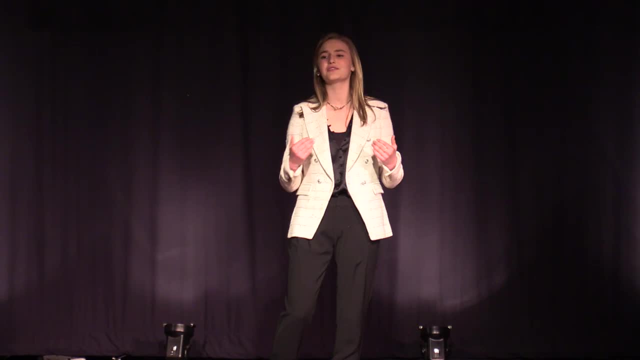 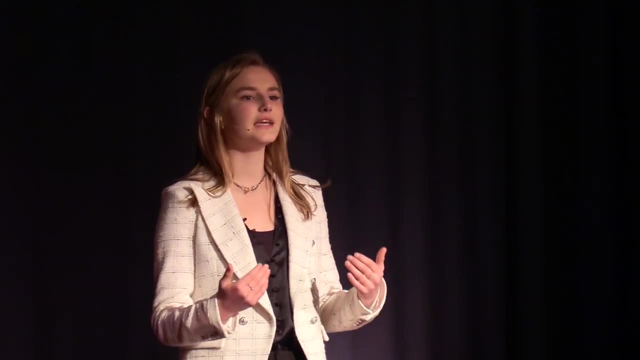 my night was going and go back to bed disappointed with the belief that, though my grades were high, my education had somehow failed me. Failed me in that it provided me with these false and early onset notions that the end justifies the mean Study and work hard for. 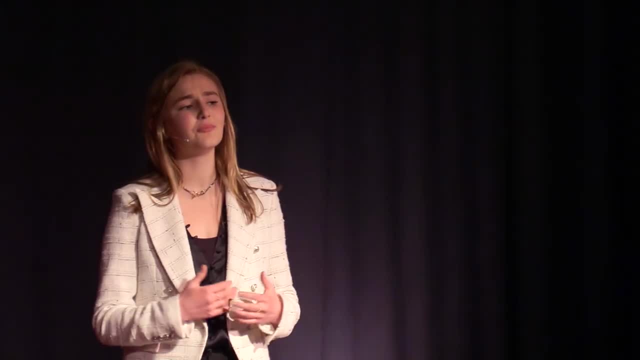 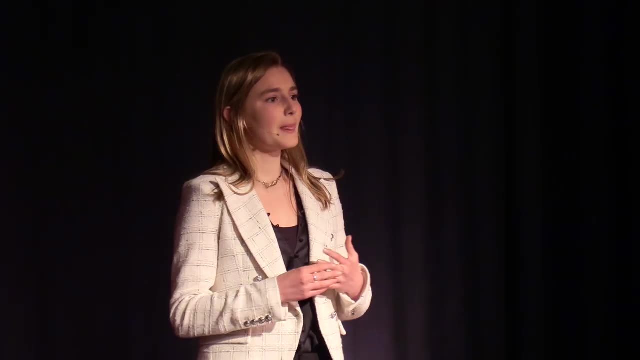 short amount of times. pull that all-nighter, get the good grade and then move on and be better because of it, right. Yet this is just not working for us. obviously You might, too, see yourself doing this, as you vow that after that next test, stressful job assignment or midterm paper, you're going. 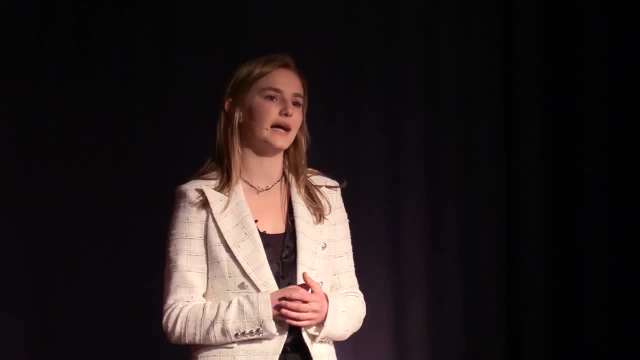 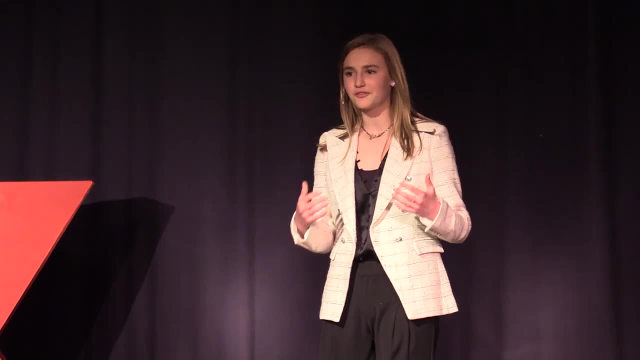 to change your ways. You're going to be more productive and you're going to waste less time. Waste less time. Oh, the amount of times I've told myself I was going to do that. But don't get me wrong, I'm all for goal setting and New Year's resolutions. After all, it 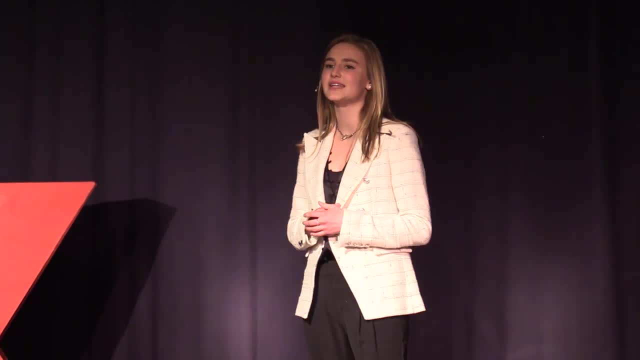 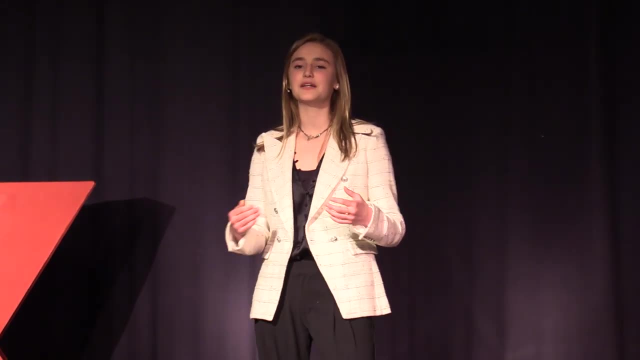 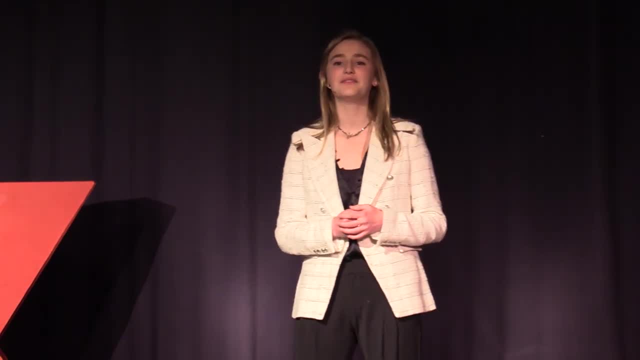 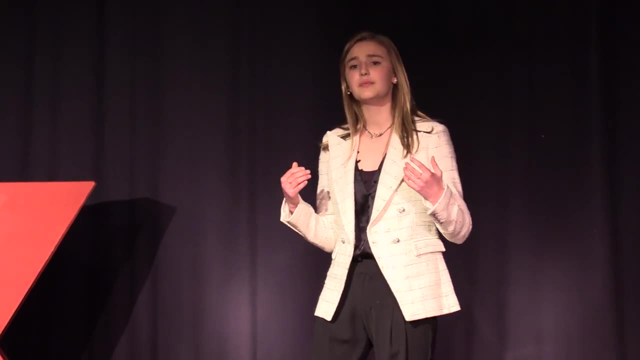 change yourself. I'm just going to let you in on a little secret you might have not already heard. It's not going to last Give yourself another stressful week, another stressful job or school assignment, and you're going to be running back to your familiar habits. 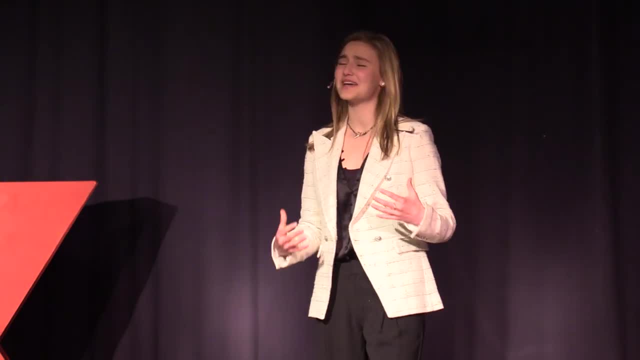 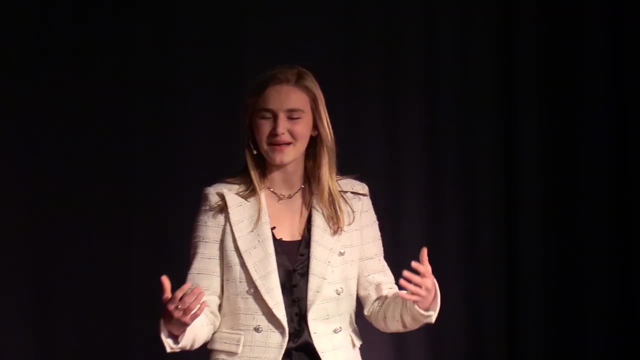 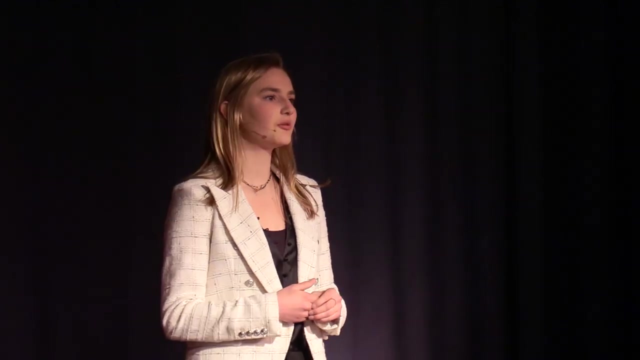 simply a single person trying to accomplish 20 things all at once and with absolutely no amount of time in the world that would ever come close to being enough. Because that's what it's about in our modern-day lives, right? We are a society composed of stressful jobs and school assignments and frantic schedules- Every single. 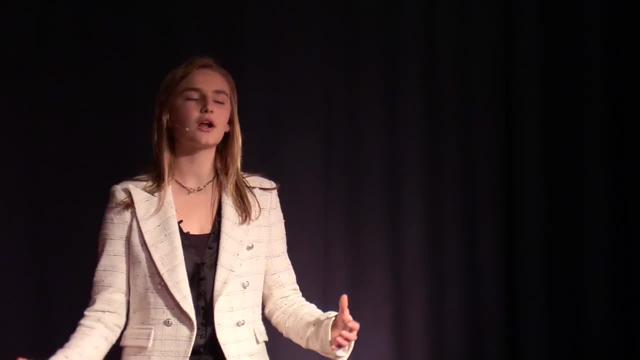 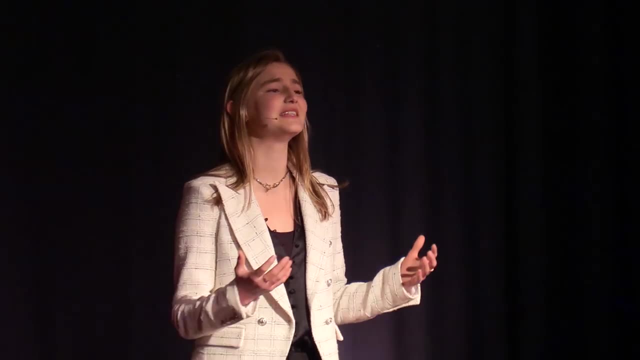 person caught in a frenzy to not only do today's work but get caught up on the mounds of work from yesterday. Because, as every person alike to me knows, yesterday always gets spent doing the work of the day before, And so it seems impossible to ever get caught up to catch. 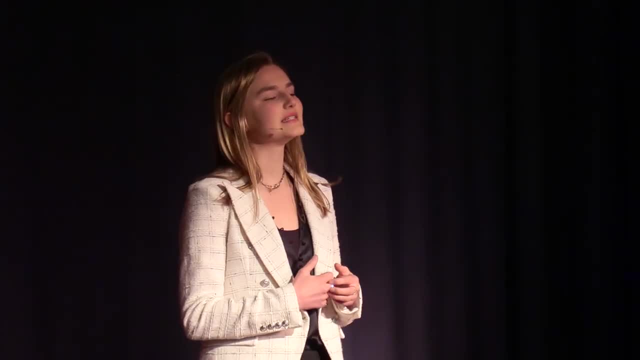 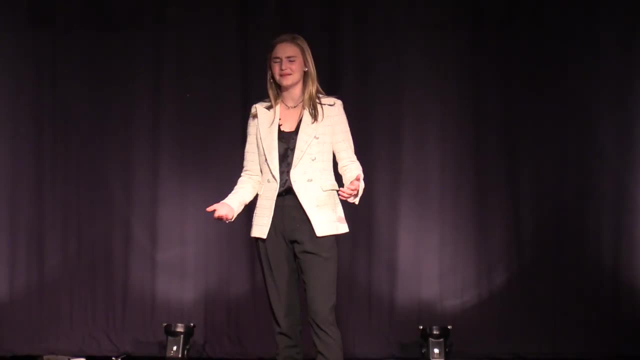 a breath without sacrifice and getting left behind, Because in today's world, time stops for no one and nothing. So is there any hope to manage time, to get a life, To get more than two hours of sleep at night? If you'd asked me a year ago, heck. 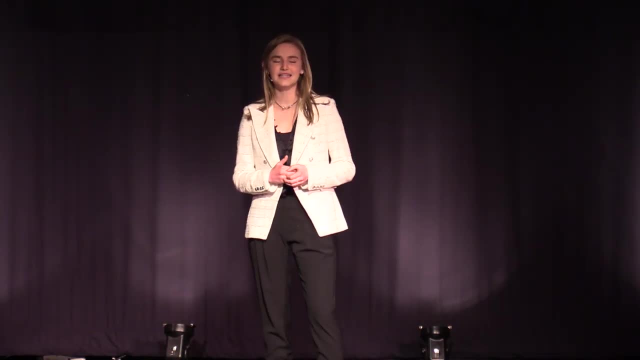 even a few months ago, I might have laughed at you and thought you were crazy, Because the most ironic part of this all was that this girl, me, the sleep-deprived woman with bags in her eyes, carrying around five gallons of Starbucks, just trying to get through the 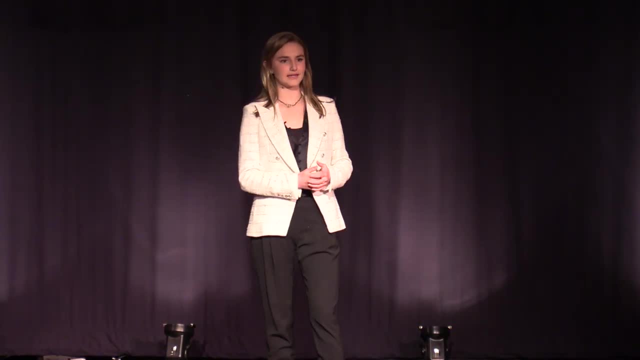 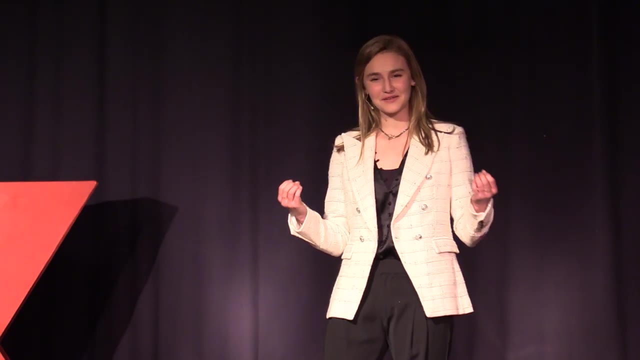 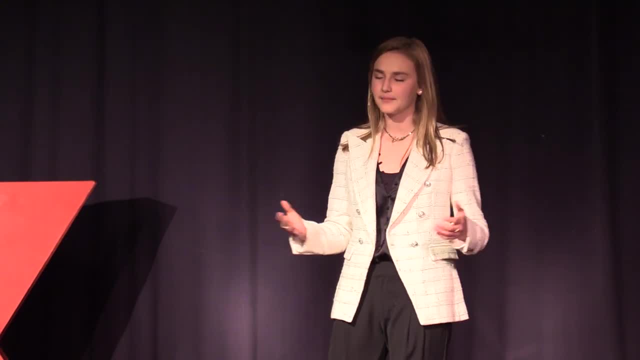 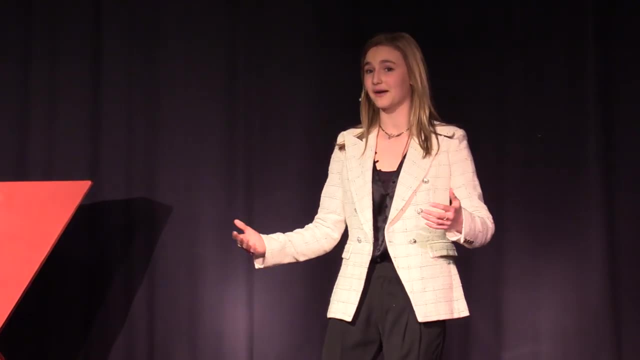 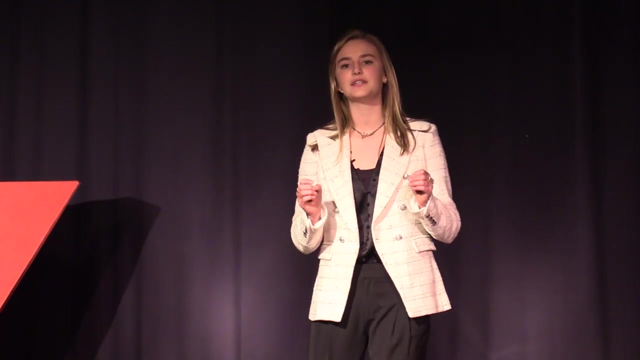 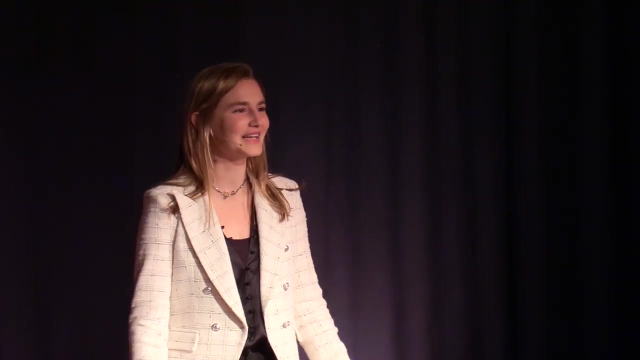 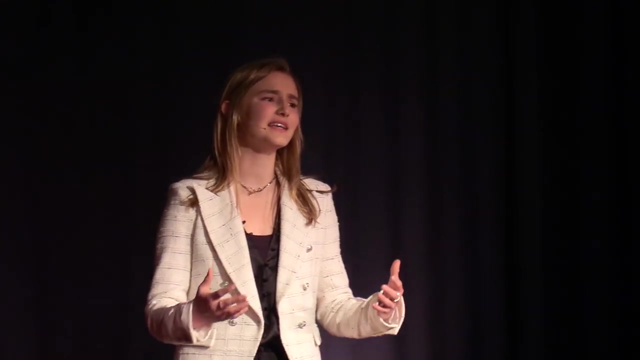 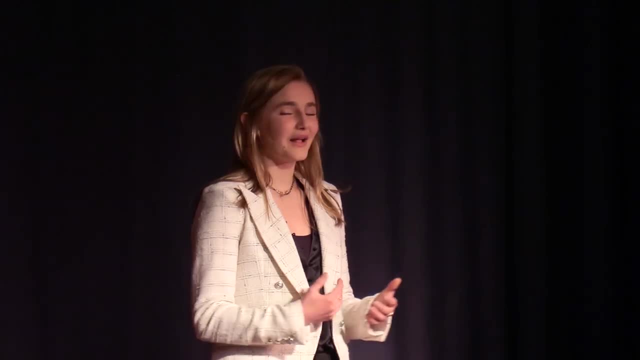 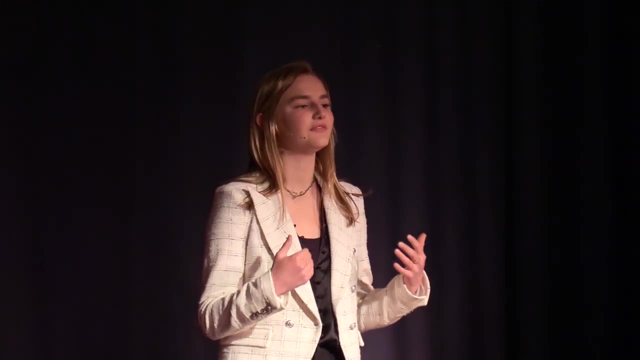 goes on and on and on. And while in theory, all these things sound so great, let's just be honest for a second. We're humans after all, and the times that we have tried and failed with time management far outweighs our success with it. I mean, have you ever noticed the growing trend of 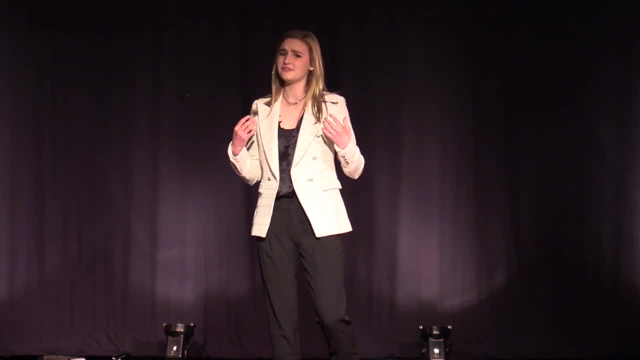 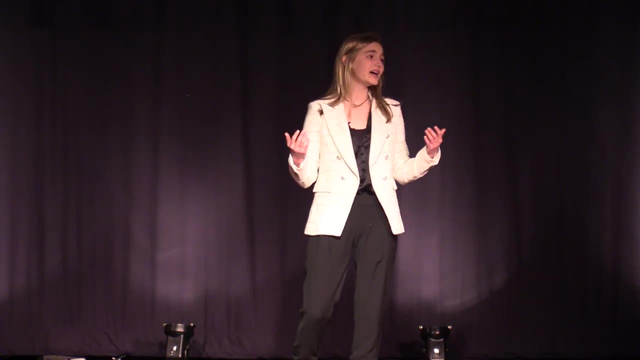 people becoming organized, appearing busy, definitely feeling busy, but at the end of the day, not accomplishing their goals. At the end of the day, coming home and saying I don't know what happened. I feel like I've been working so hard for so long and have nothing to. 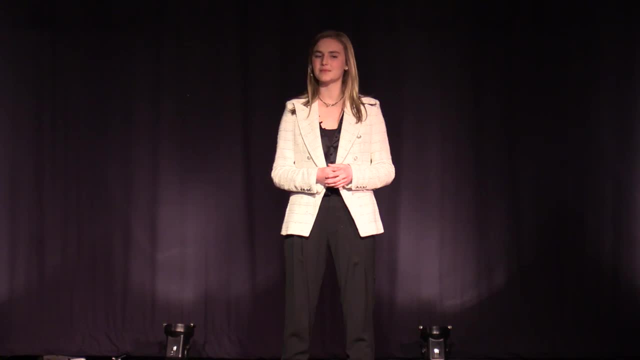 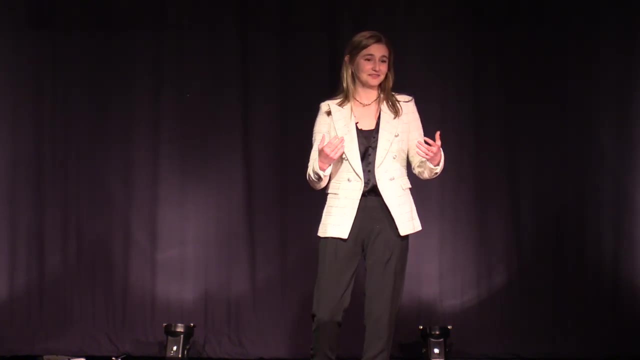 show for it. So what if time management is not, in fact, the cure to all of our problems? I mean, if the end goal to time management is to have some more downtime and not feel so behind at work, why do we still feel so pressed for time all of the time? 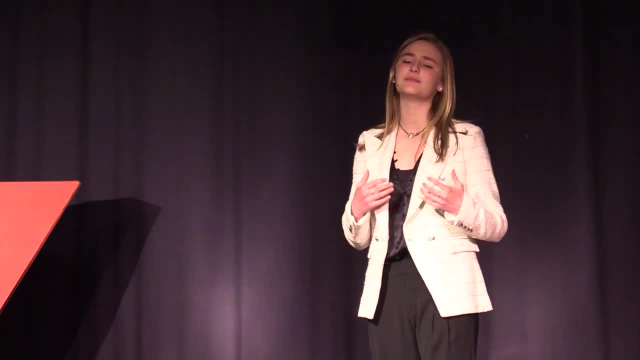 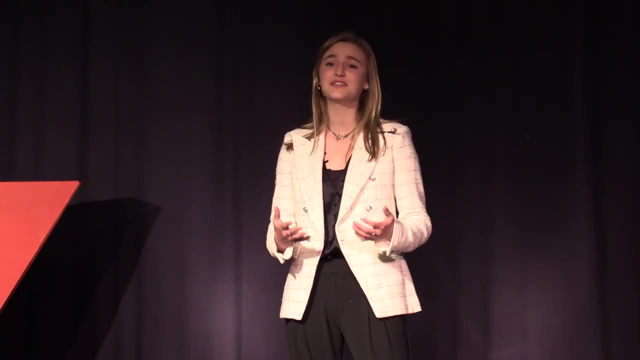 Why have the words I feel so behind? there's just not enough time. I'm so stressed Become the new daily chant of every single student, parent, teacher, employee, intern supervisor and boss all alike. I hate to break it to you, but time management is simply not. 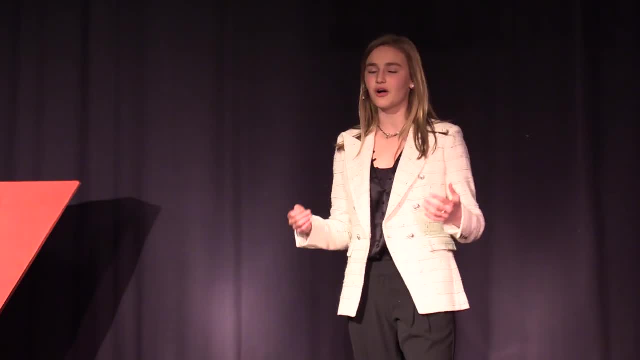 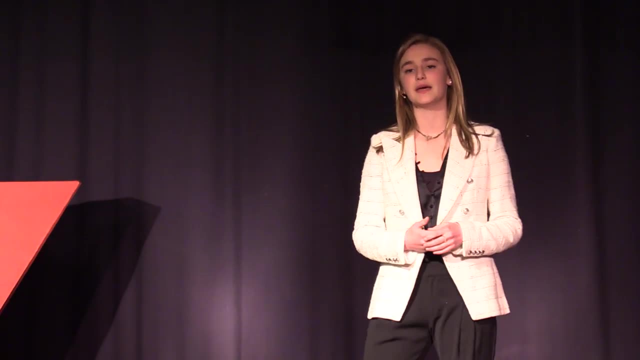 working for us. It is masking itself as a solution to all of our problems, when, in reality, it is only further propagating, the true issue at hand being our lack of self-management. My friends, the problems you're experiencing is not because of your inability to follow along with the set. 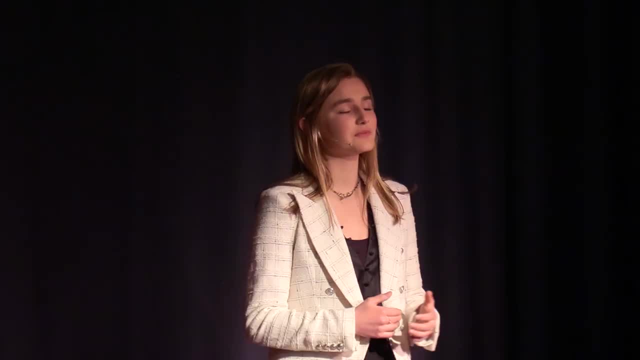 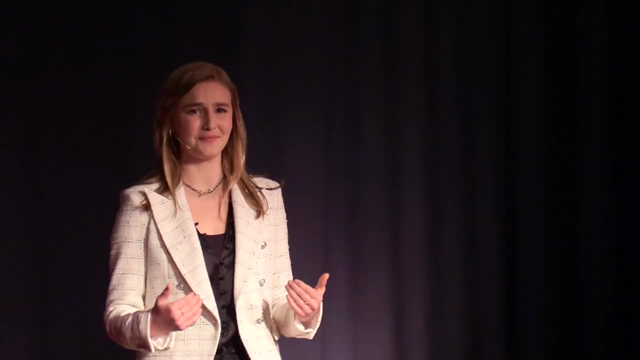 procedures of time management. It is because of your inability to follow along with the set procedures of time management. It is the fact that time management in of itself is fundamentally flawed. Someone please explain to me how we think we could possibly manage time. We can't alter it. 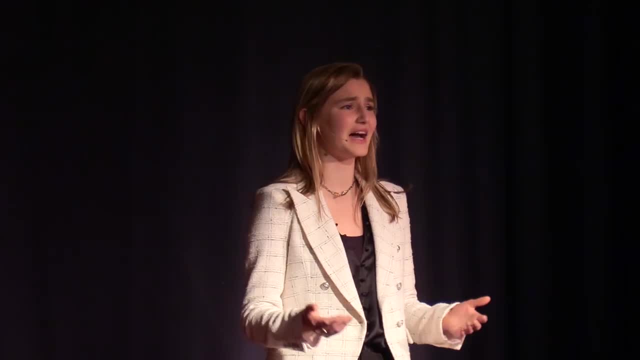 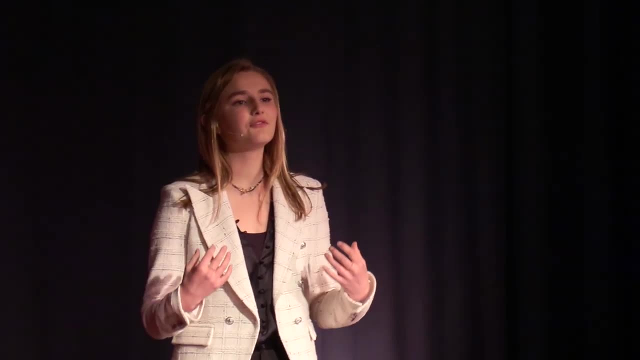 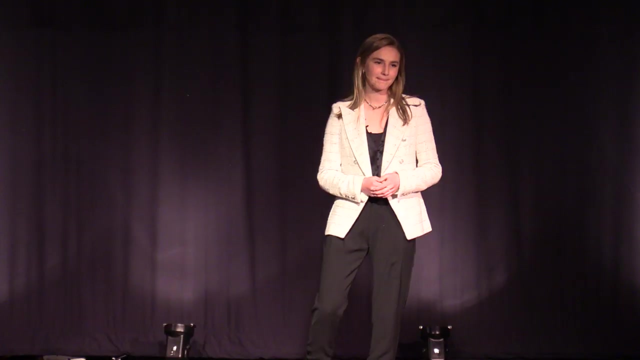 we can't make it go slower or faster, We can't divvy it up and save little tidbits here and there for our pleasing. And, moreover, our attempt to configure time and form it into such a thing that can be coordinated and controlled to the very last second only drives us crazy. I know that this is. 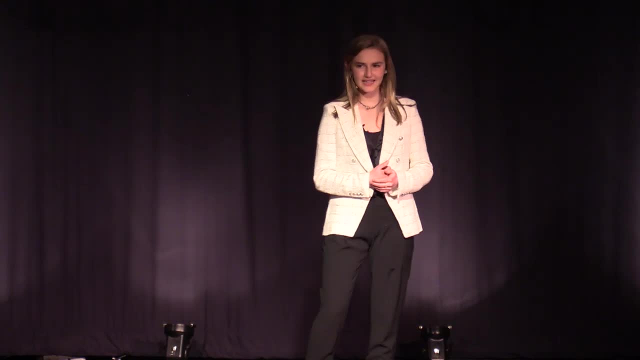 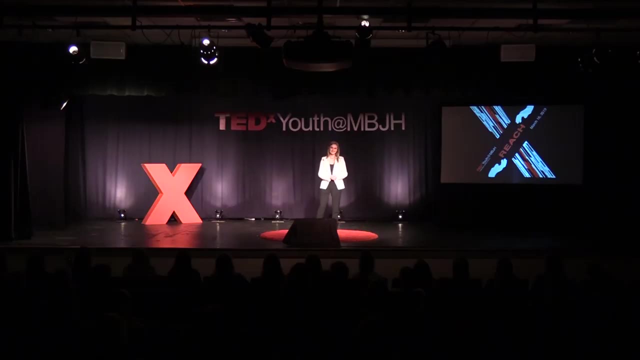 probably never happened to any of you guys, but has anything ever not gone according to plan? Has life ever actually gotten in your way of your perfectly organized day? I know crazy right, How dare it? But, in all seriousness, when we rely on these perfectly time-managed days and something, 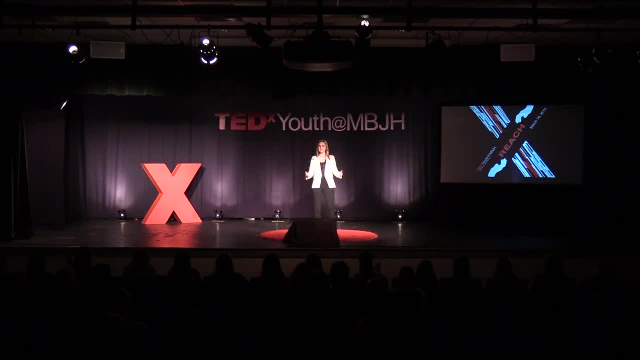 doesn't go according to plan, we find ourselves entirely unable to handle the situation, paralyzed with fear and stress and every other emotion entirely non-existent. We're not able to handle it. We're not able to handle it. We're not able to handle it. Time management techniques do not. 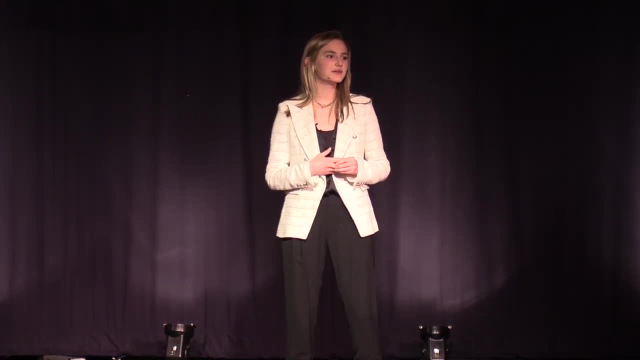 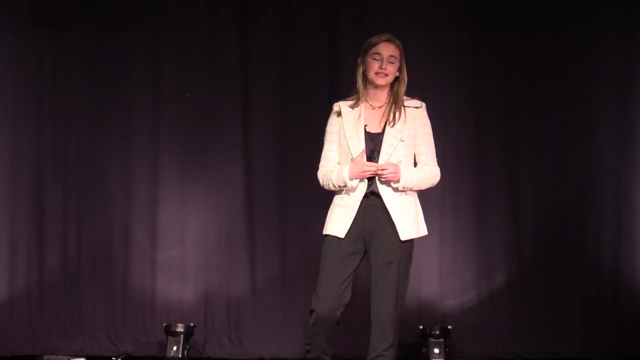 take into account the imperfections of daily life, the ensuing chaos of a day that doesn't go according to plan, In other words, the chaos of everyday life. It's just not working for us, It's not working for me, It's not working for you, And so I ask you to instead consider: 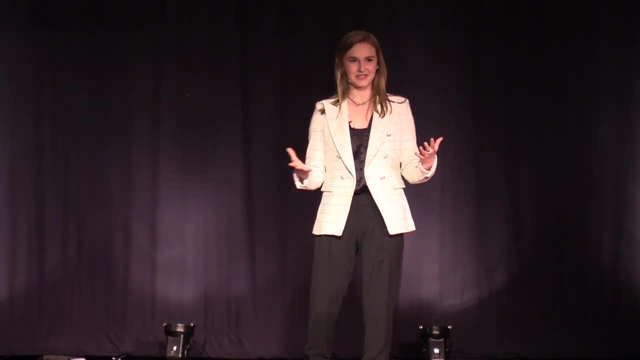 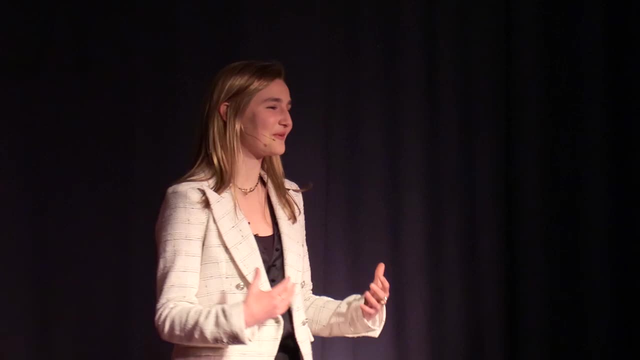 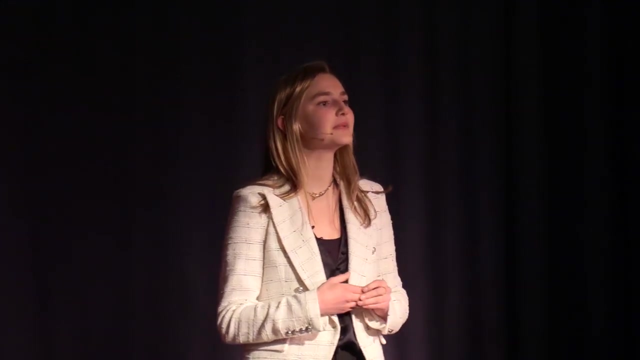 self-management. And now each one of you nods your head in perfect harmony at this entirely ambiguous term, whose cryptic meaning you're supposed to immediately understand. No, before you get worried that I'm just replacing one flawed idea with another, let me explain. Self-management is simply defined as a combination of behaviors that describes how one 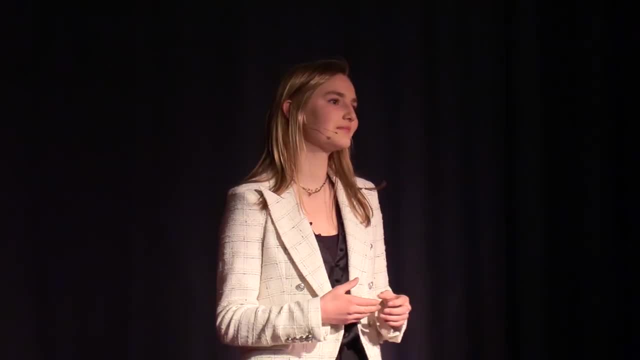 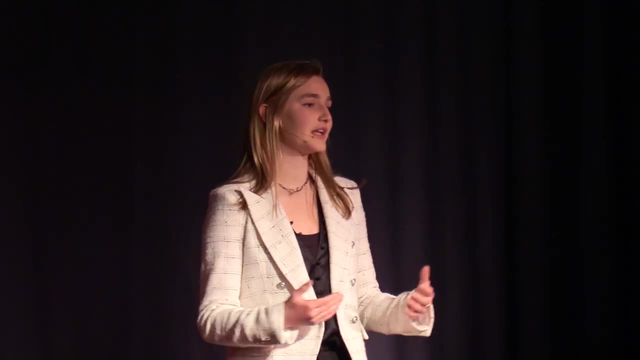 manages himself in their workplace and in their life. So, first off, it's just as applicable to the five-year-old girl starting her first year in kindergarten as to the six-year-old man in his 30th year at the corporate position, And it's also something that both of them can improve upon. It's 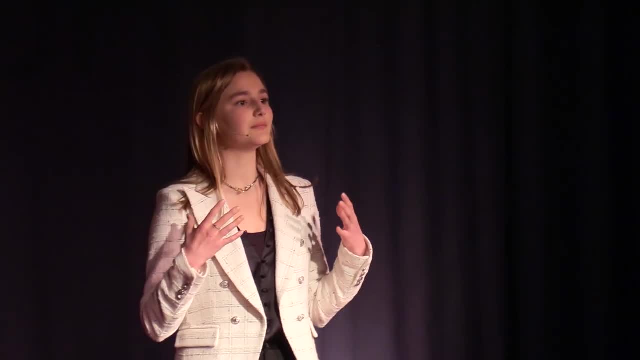 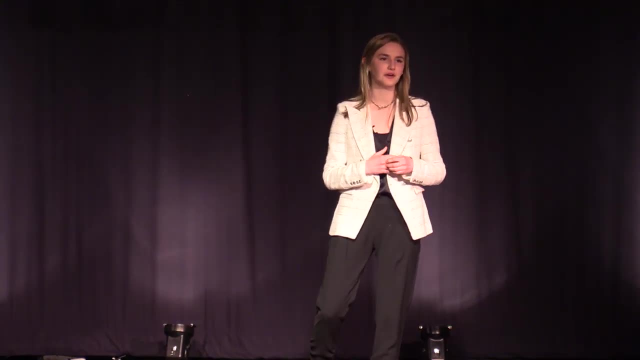 a skill that is developed throughout one's life. It's a skill that is developed throughout one's life and is designed to be to change throughout one's life and in their stage in life. One of the most important factors of self-management is the art of focus. Just because I sit down and try to